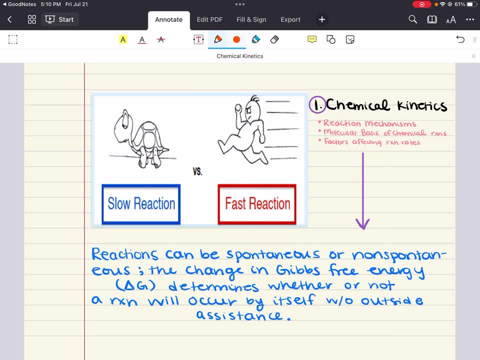 understanding the mechanisms by which reactions can occur, the factors that influence these rates, the energy transferred during reactions, and just how different variables are going to contribute to the rate of a reaction. Now, to begin to understand this, we're going to first have to 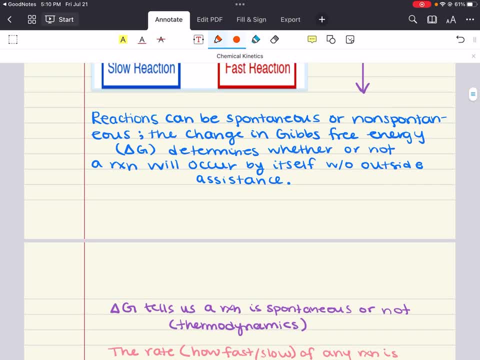 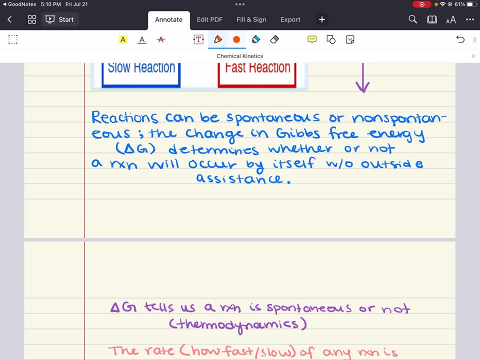 talk about Gibbs energy. All right, we're going to have to talk about Gibbs energy, also known as Gibbs free energy. This is a measure of the amount of energy that will be available to do work in a chemical system. It takes into account both enthalpy, which is the heat content. 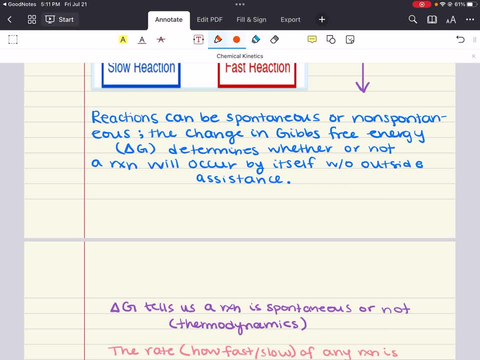 and entropy, which is the degree of disorder of a system, And it's going to be used to determine whether or not a reaction will occur spontaneously under certain conditions. Now the equation for Gibbs free energy. we cover this in previous chapters in MCAT general chemistry. They'll 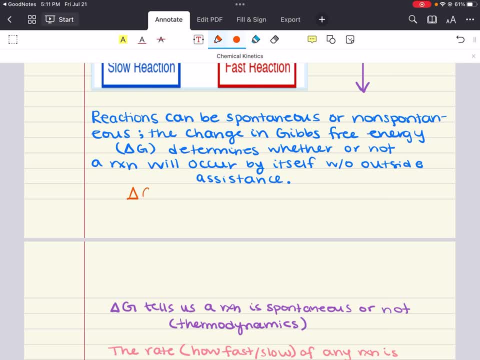 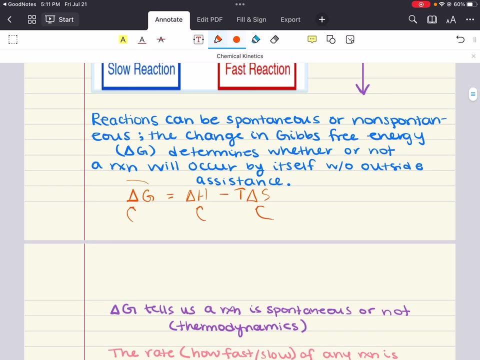 reappear later in other segments as well. But delta G change in Gibbs free energy is equal to delta H changes in enthalpy, minus T delta S changes in entropy. So reactions based off of your value for Delta G. all right, we'll tell you. it's going to tell you for. 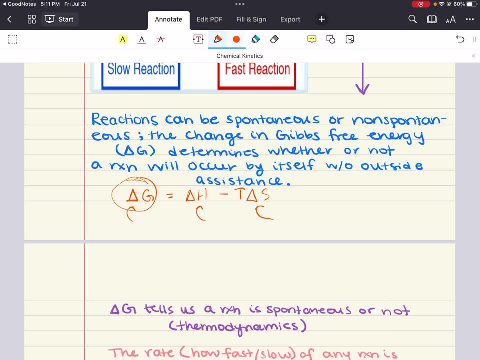 reaction- Speaker 1- or non-spontaneous. The change in Gibbs free energy delta G is going to determine whether or not a reaction will occur by itself, aka spontaneous, all right, without outside assistance, or it's going to need- quote unquote- outside assistance to proceed, So that'll be non-spontaneous. 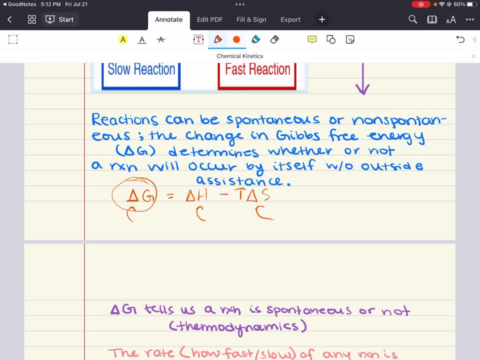 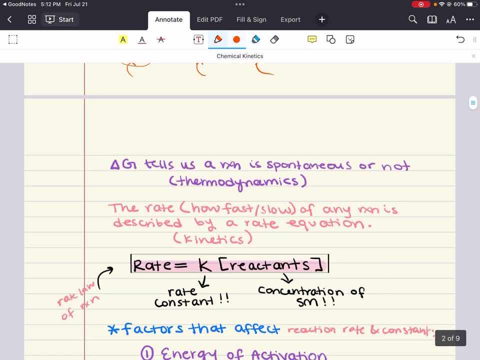 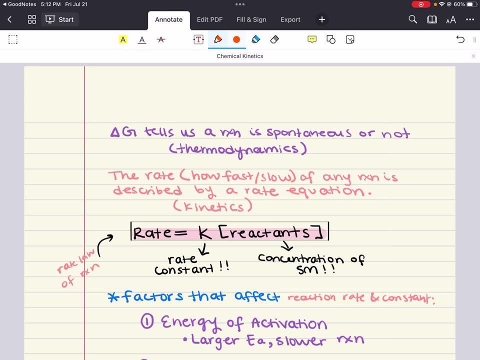 All right Now. even if a reaction is spontaneous, that does not necessarily mean that it's going to run quickly. In fact, nearly every biochemical reaction that enables life to exist, while it is perhaps spontaneous, proceeds so slowly that, without the aid of enzymes and 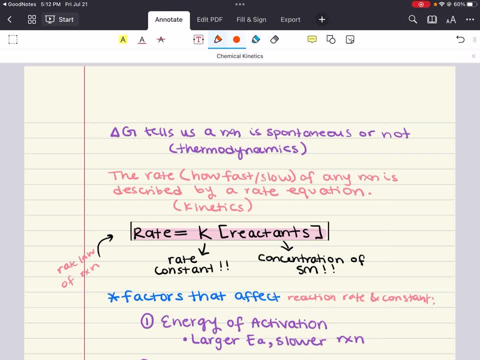 other catalysts, measurable reaction. progress might not actually occur over the course of an average human life. all right, So now an important distinction needs to be made here. all right, And that important distinction is that we need to understand the difference between thermodynamics and kinetics. all right, 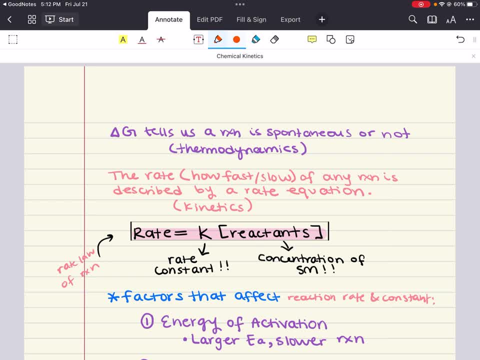 Thermodynamics is concerned with the energy changes that occur during a chemical reaction. On the other hand, kinetics is concerned with the rate at which reactions occur. So, in other words, thermodynamics deals with whether or not a reaction will occur, while kinetics deals. 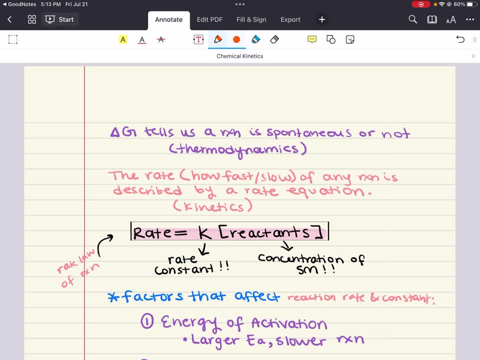 with how quickly that reaction will occur. all right, Thermodynamics can tell us whether a reaction will occur at aada or not, and thermodynamics can tell us how quickly that reaction will occur is energetically favorable, but it cannot tell us anything about the rate at which the reaction 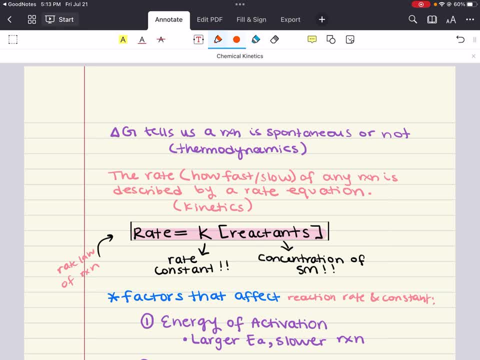 will occur. all right, That's what kinetics is for. So that means change in Gibbs. free energy will tell us if a reaction is spontaneous or not, while the rate of any reaction is going to be described by a rate equation which gives us kinetic information. So that distinction is. 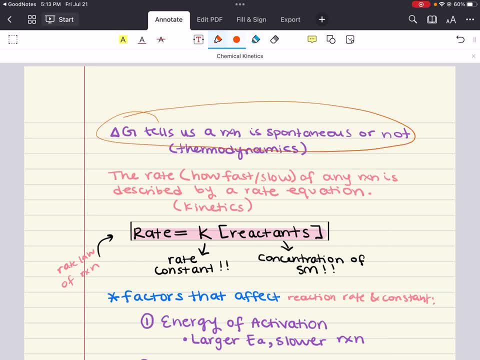 really important. all right. Delta G tells us if a reaction is spontaneous or not. This deals with thermodynamics. We had a whole chapter on thermodynamics already as well. all right, But then if you want to know the rate of a reaction, is it going to be a fast reaction, slow reaction? 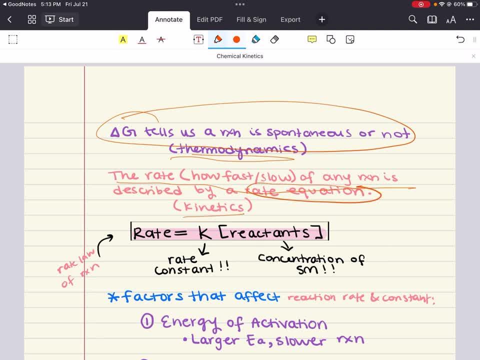 that's going to be described by a rate equation, which we're about to get into, and that's all kinetics. Now, as we're going to see shortly in more detail, shortly, all right, a rate equation is an equation that describes the rate of a reaction, and that's all kinetics. 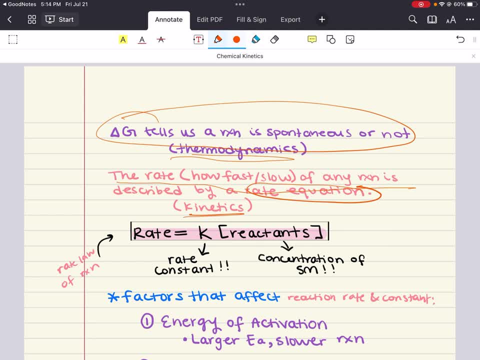 It describes how the rate of a chemical reaction depends on the concentrations of the reactants, and the general form of a rate equation is the following: Rate is equal to K, which is a rate constant all right, multiplied by the concentrations of the reactants or the starting. 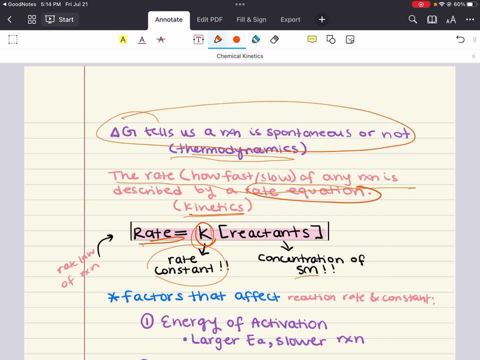 material, all right. Now it's going to have a more detailed form, right? You can have K, all right. and if you had two reactants, say A and B, all right, then your rate will be your rate constant multiplied by the concentration of A. 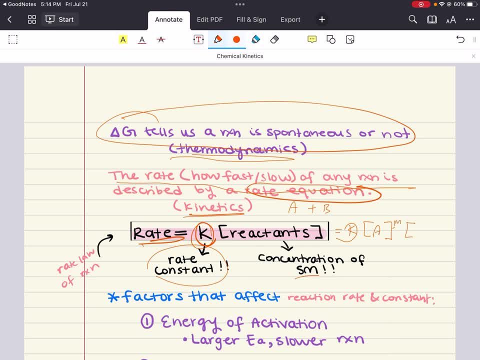 to some specific order. we'll talk about this shortly. multiplied by your other reactant B, all right, that also has some sort of reaction order, all right. So a rate equation is an equation that describes how the rate of a chemical reaction depends on the concentrations of the. 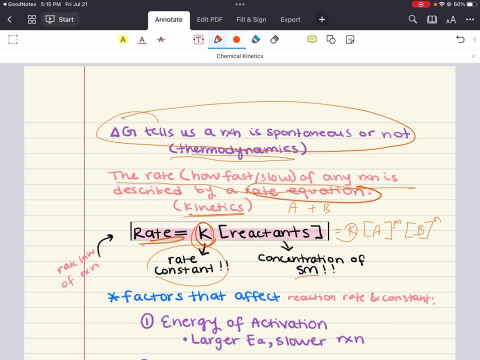 reactants. We're going to go and see how that works, and we're going to go and see how that works in so much more detail here shortly, all right, So just hold on. all right, We're going to take that definition. we're going to elaborate on it. Now there are several things that are 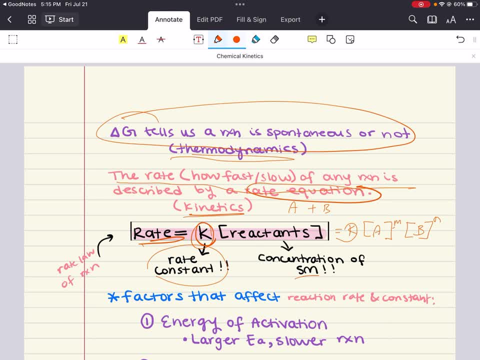 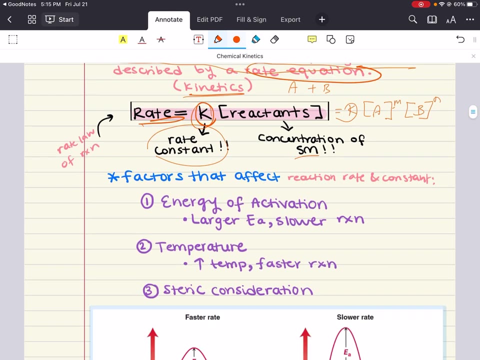 going to affect your rate constant. there are several things that are going to affect your rate of reaction, all right, And so we want to talk about several factors that are going to affect essentially the kinetics of a reaction. all right, First thing that we want to talk about. 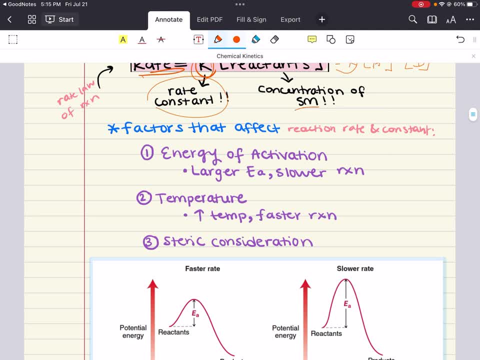 is your activation energy. All right, Your activation energy is the minimum amount of energy that's going to be required for a chemical reaction to occur. In order for a reaction to take place, reactant molecules are going to have to collide with sufficient energy. 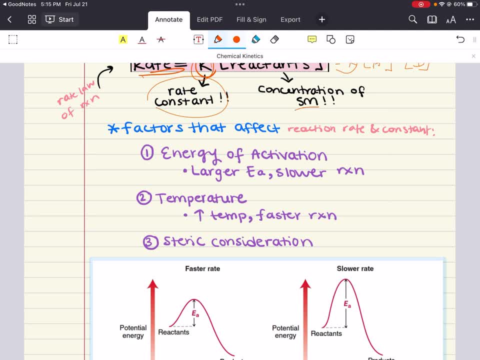 all right to overcome some activation energy barrier. The higher the activation energy, the slower the reaction rate, because fewer molecules will have sufficient energy to react. On the other hand, a lower activation energy means that more molecules will have sufficient energy to react. 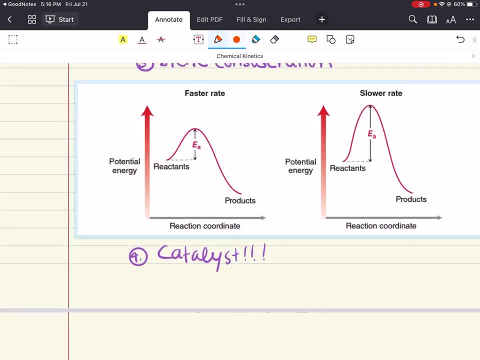 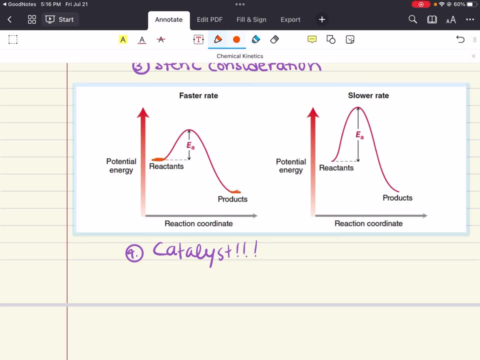 resulting in a faster reaction. So, for example, if we look at this diagram here, all right, here's where you're starting off with your reactants. here are your products. To get from reactants to products, you have to overcome some activation energy. Notice how this. 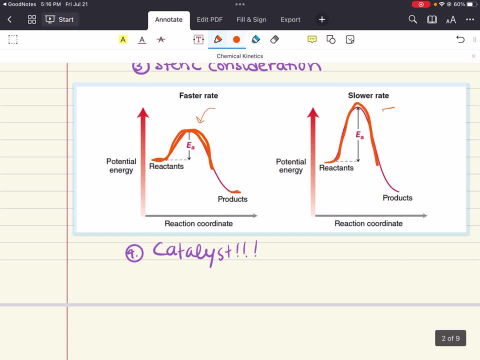 activation energy. compared to say this activation energy right here, all right, one is smaller than the other. So this one, I'm going to say, is going to be smaller than the other. So this one right here is smaller. This is going to have a faster rate than this reaction which has a larger 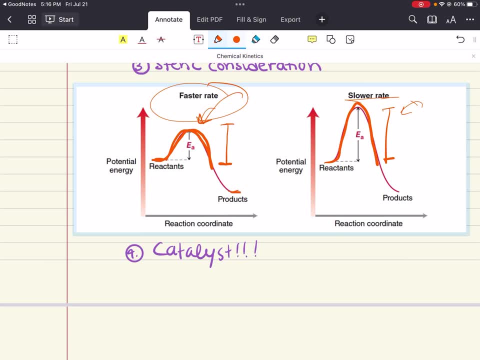 activation energy. It's going to have a slower rate generally, all right. So activation energy is one thing that's going to affect the kinetics of your reaction. Now you can overcome a higher activation energy using something called a catalyst, which can affect your kinetics as well. 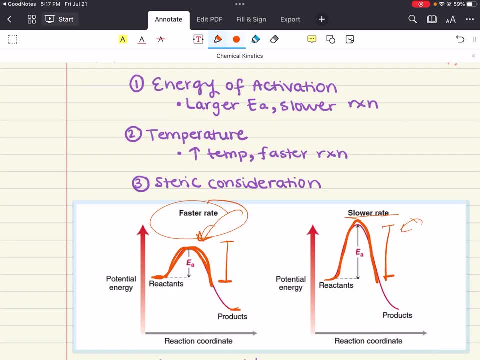 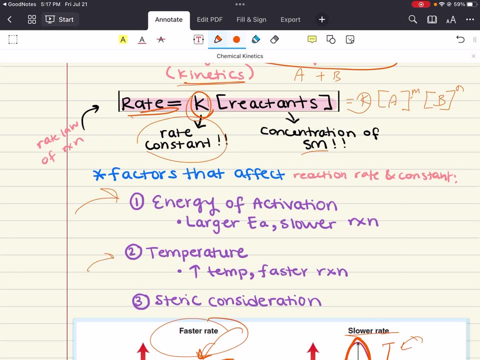 We're going to talk about that here in like three points, all right. So activation energy is one thing that can affect your kinetics- All right. another thing that can affect your kinetics is temperature. all right, For nearly all reactions, the reaction rate will increase as the temperature increases. Now, because the 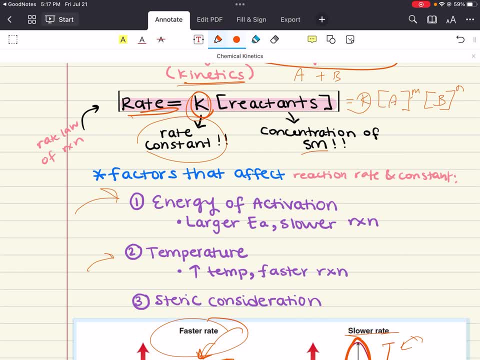 temperature of a substance is a measure of the particle's average kinetic energy. increasing the temperature is going to increase the average kinetic energy of the molecule and, as a consequence, the proportion of reactants gaining enough energy to, say, surpass the activation energy. 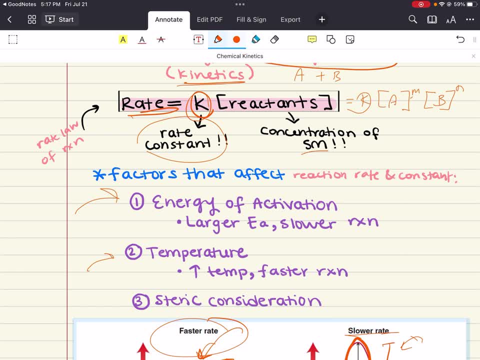 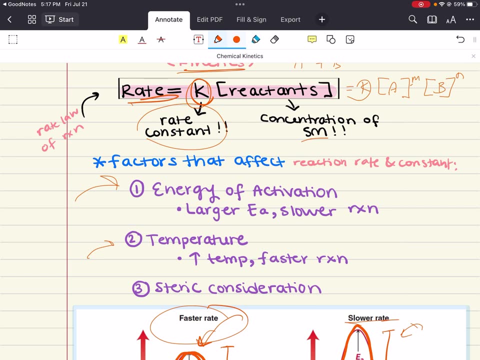 and therefore capable of undergoing a reaction, is going to increase with higher temperature. Now you're going to often hear that raising the temperature of a system by 10 degrees Celsius will result in an approximate doubling of the reaction rate. all right, That is sometimes true. 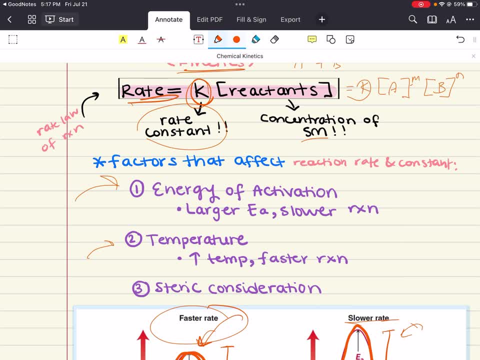 but just be careful with this approximation right, Because while it is generally true for biological systems- all right, it might not be so true for many other systems. So if you're a biologist, you have to remember that even in biological systems, if the temperature gets, 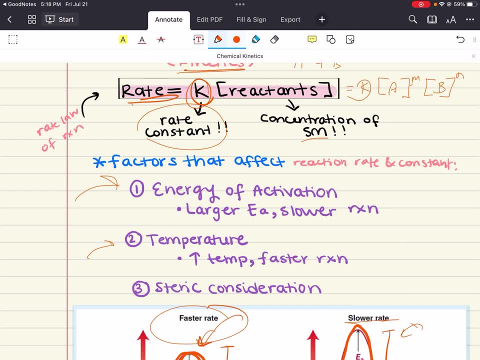 way too high, all right. then an important catalyst may denature and the reaction rate could reach a barrier where it just plummets, all right. So keep that in mind moving forward. Another thing that can affect your kinetics is steric considerations. all right, Steric. 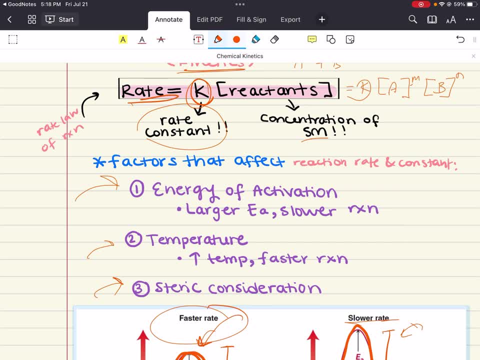 considerations can play a role in determining the temperature of a substance. So if you're a biologist, you can determine the temperature of a substance by determining the rate of a reaction, by affecting the likelihood of reactant molecules colliding with one another in a way that will allow for. 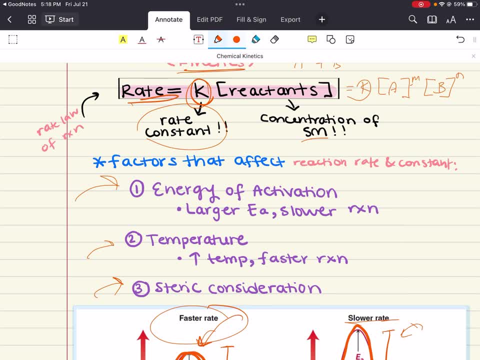 the reaction to occur. So, specifically, if there are steric hindrances, all right. steric hindrances can reduce the rate of a reaction by making it more difficult for reactants to come into close proximity with one another. And this is because, say, a large bulky substituent can. 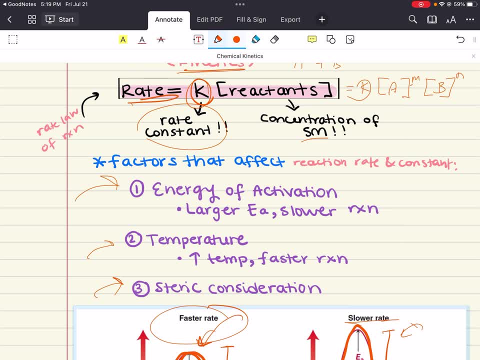 create steric hindrances. So if you're a biologist, you can determine the temperature of a substance and that could prevent reactants from getting close enough to form the necessary bonds for the reaction to proceed all right As a result. reactions involving large substituents: they may. 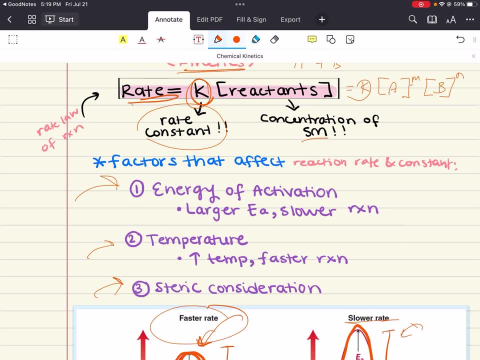 proceed more slowly than reactions involving smaller substituents. So the size of your substituents, steric considerations, are things you need to keep in mind as well when you're thinking about what could affect the kinetics of your reaction. all right, What could affect? 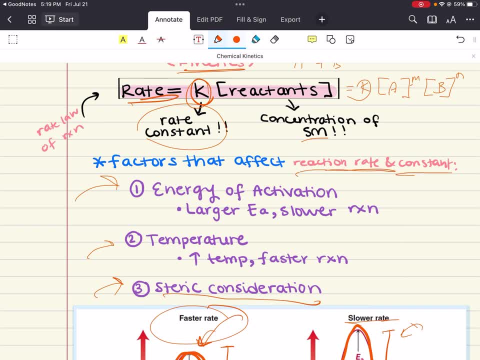 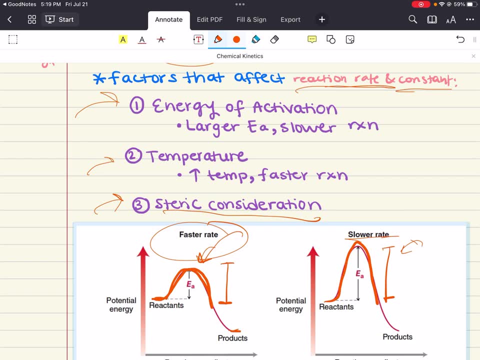 your reaction rate and your reaction constant, your rate constant, all right. Now, on that note, you can also consider reactant concentrations. all right, steric considerations, but you can also consider here reaction concentrations, all right, The greater the concentration of reactants. 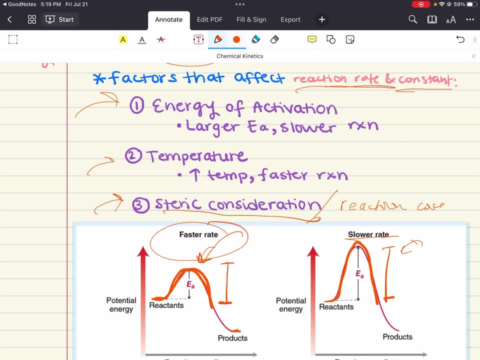 the greater the number of effective collisions per unit time, And so, therefore, the reaction rate will increase for all but one. So if you're a biologist, you can determine the temperature of zero order reactions, which we're going to discuss shortly. all right, Last but not least. 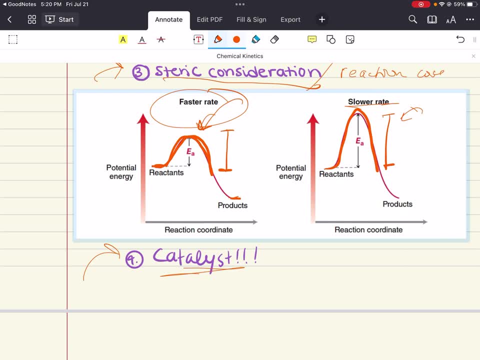 another factor that affects reaction rates and your constants is your catalysts. Catalysts are substances that increase reaction rate without themselves being consumed in the reaction. Catalysts interact with the reactants, either by absorption or through the formation of intermediates, and then they stabilize them so as to absorb the reactants. So if you're a biologist, 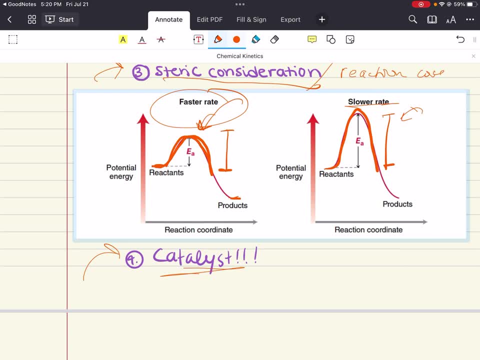 to reduce the activation energy necessary for the reaction to proceed. Now, while many catalysts, including all enzymes, chemically interact with the reactants, they're going to return to their original chemical state after formation of the product. Now they may increase the frequency. 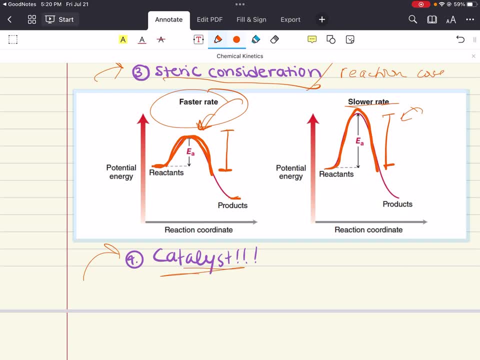 of collision between the reactants. They could change the relative orientation of the reactants, making a higher percentage of collisions effective, or they could donate electron density to the reactants or even reduce intramolecular bonding within reactant molecules. All those are. 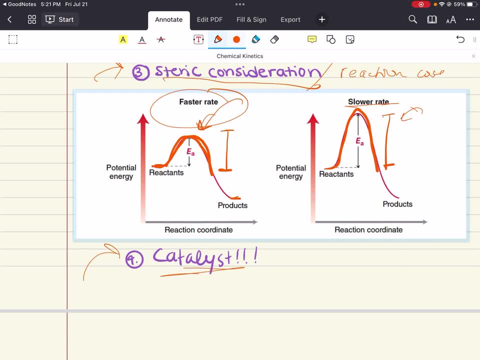 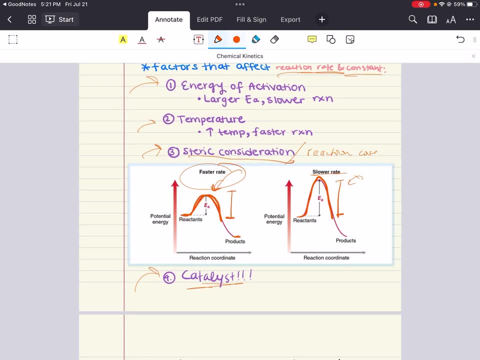 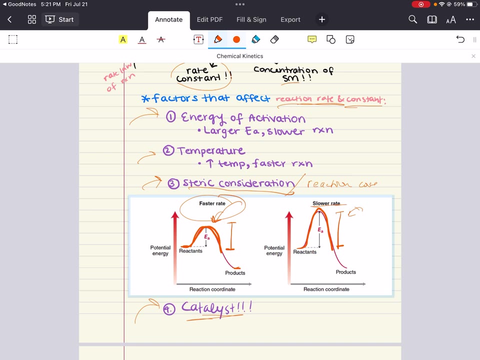 possible actions of catalysts that are going to help in speeding up reactions. all right, So with that we've covered a couple of factors that are going to affect your reaction rate and your rate: constant energy of activation, temperature, steric consideration, reaction. 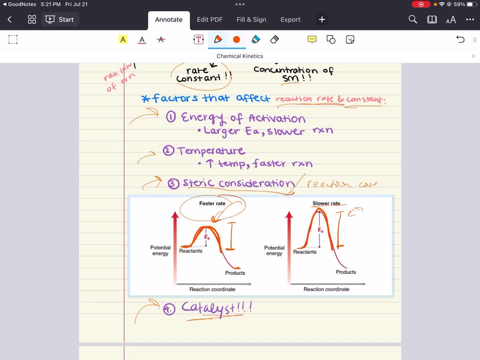 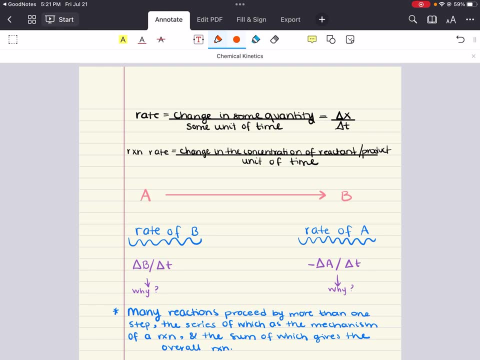 concentrations and catalysts. With that, let's just take a quick step back, all right, and really define the word rate. okay, The word rate Rate is a change in some quantity, all right, over some unit of time You can write. 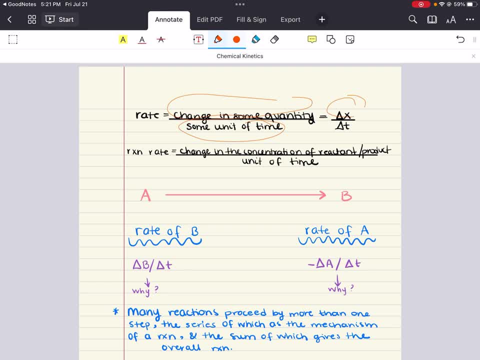 this as delta x over delta t. all right, Some change a change in some quantity over some unit of time, Specifically here, when we talk about rate. all right, we're discussing a reaction rate. So what we're saying is: 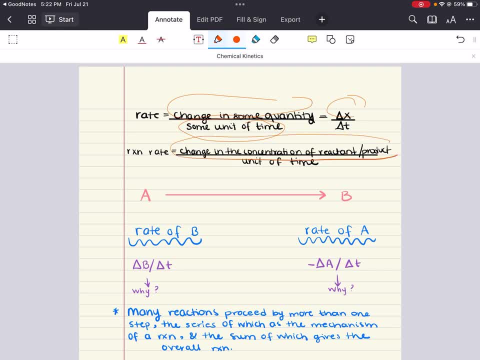 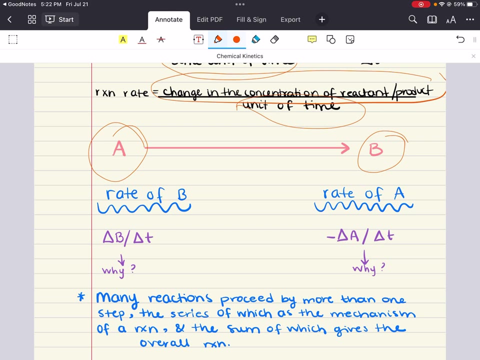 change in some quantity will actually be change in the concentration of reactant or product over change in unit of time. Now if we consider a generic reaction going from reactant A to product B- all right, where one mole of B can be produced from one mole of A, well we can describe the rate. 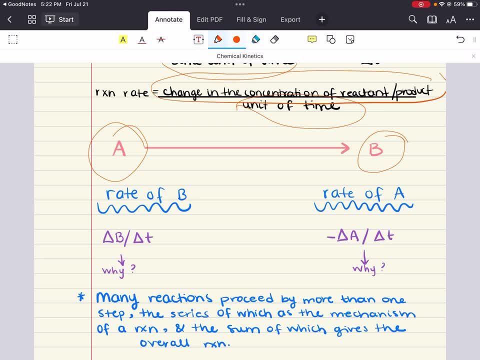 of this reaction in terms of either the disappearance of reactants over time or the appearance of products over time. okay, Because the reactants, by definition, are being consumed in the process of formation of the products. all right when we talk about. 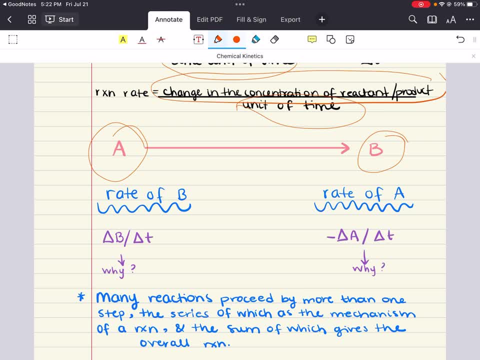 the rate of the reactants. we place a negative sign all right in front of the rate expression for the reactants, all right. So the rate of A is going to be minus change in reactants over change in time, And that's because we're consuming reactants over time. So we're consuming reactants. 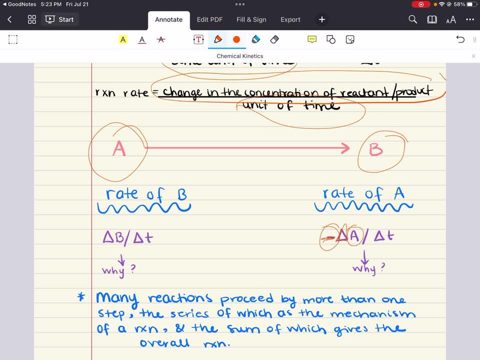 over time. So we're consuming reactants over time. So we're consuming reactants. reactants are being consumed throughout this reaction to form the products, all right. Similarly, we can write the rate of reaction for product B: right, It's being formed and so there's a positive sign, all right. 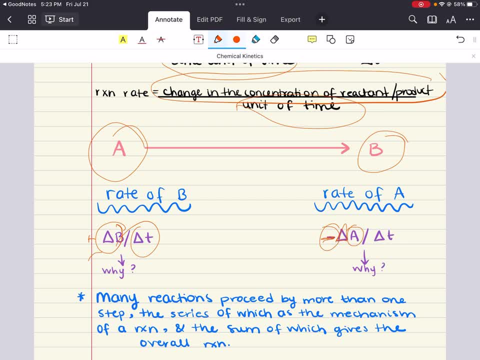 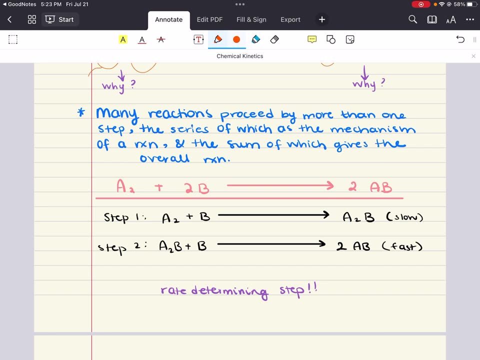 change in B over change in time. all right, Now, this is a simple: one reactant, one product reaction. We're going to build on this definition here in a little bit. Now, very rarely we're going to is the balanced reaction equation. you know that's used for determining limiting reactants. 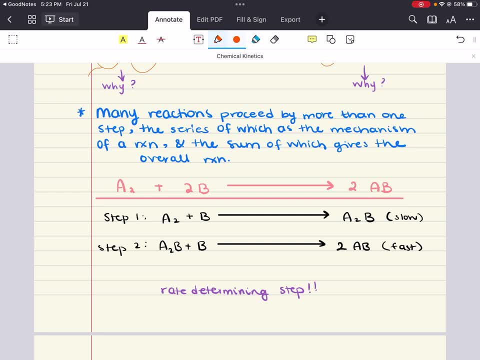 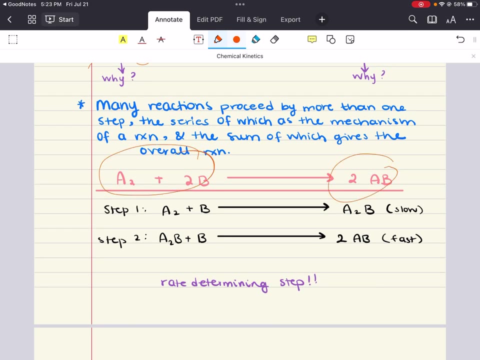 and yields an actual, accurate representation of the steps that are involved in the chemical process, from reactants to products. Many reactions, right, you're going to see. here's the reactants. all right, Here are the products. Many reactions, though, are going to proceed. 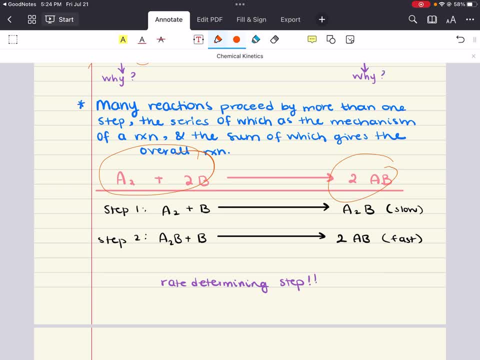 by more than one step. all right, They're going to proceed by more than one step. They're going to proceed by more than one step, the series of which is known as the mechanism of the reaction, and actually the step of all those. the sum of all those steps gives you this overall. 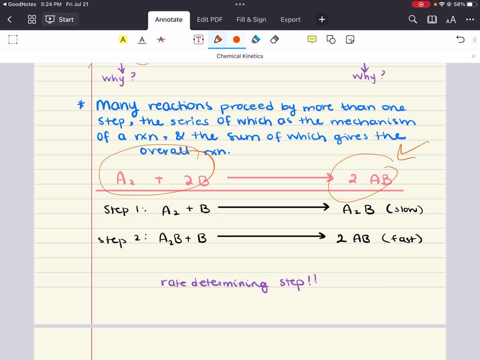 reaction that you see all right. So, knowing the accepted mechanism of a reaction, it might help explain the reaction's rate, the position of equilibrium and even thermodynamic characteristics. So if we're looking at a reaction like this, right the very 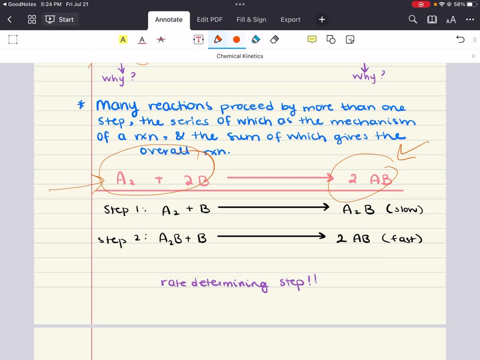 a possible reaction you might see. you might encounter, all right, some reactant plus this other reactant form, this product. all right, This is a form of a reaction that you might see. all right, a generic reaction On its own. this equation seems to imply a mechanism in which 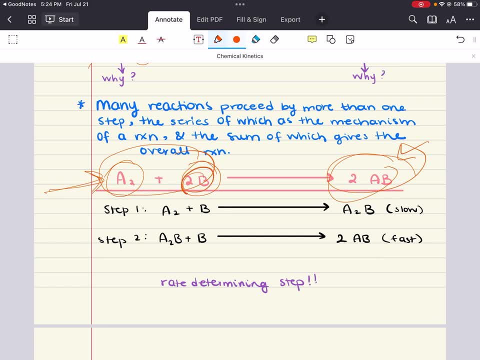 two molecules of B collide with one molecule of A2 to form two molecules of product A- B. all right, But again, many reactions, they proceed by more than one step, which you don't necessarily see in this general generic reaction form. Suppose instead, however, that the reaction 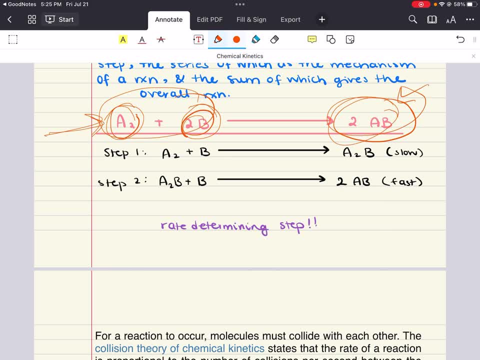 okay, it's going to take place in two steps, all right. Let's look at what those two steps are that give us this generic reaction. all right, And note that the two steps taken together are going to give the overall reaction. So let's look at what those two steps are that give us this generic 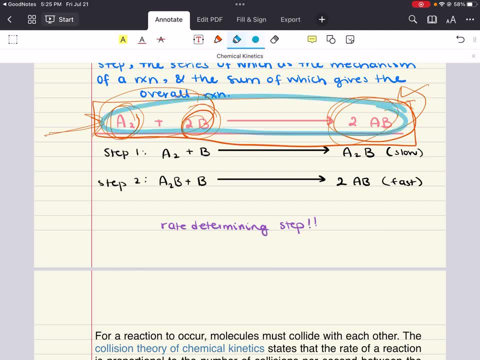 reaction. all right, that we see given to us here, all right. So we start off with step one. all right. The molecule A2 plus B first gives us this product A2B, all right, And then in step two, 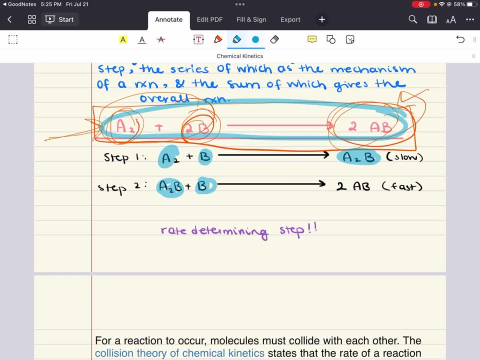 we have that A2B plus some more of that reactant B to give us our final product 2AB. all right, Note that this molecule A2B. all right, it does not appear in this reaction that we see, in this overall reaction that we see here. This A2B molecule is called. 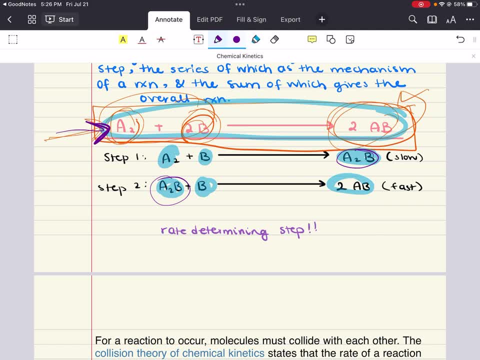 an intermediate, all right. Reaction intermediates are often difficult to detect because they may be consumed almost immediately after they're formed. But a proposed mechanism that includes intermediates. it can be supported through kinetic experiments. One of the most important points to remember here, all right, is that in a process like this, where there's two steps, that 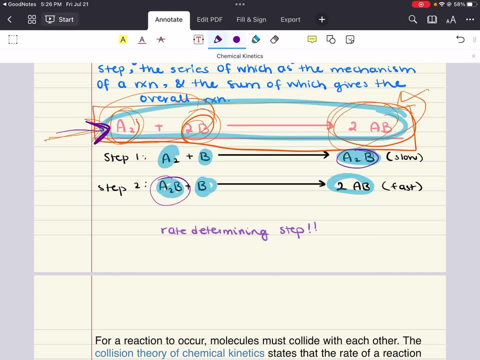 are happening. all right, the slowest step in a proposed mechanism that's going to be called your rate determining step, because it acts like a kinetic bottleneck preventing the overall reaction from proceeding any faster than that slowest step. So let's look at step two. So let's look at 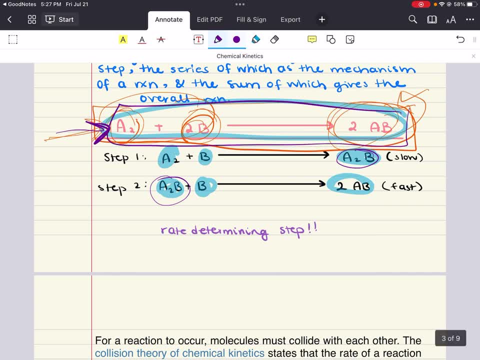 step three. So for this overall reaction we saw that it involved two steps. One of these molecules that's formed is not seen in the overall net reaction. all right, And that's because it appears as a product in one step and as a reactant in the other step. all right, And so it technically 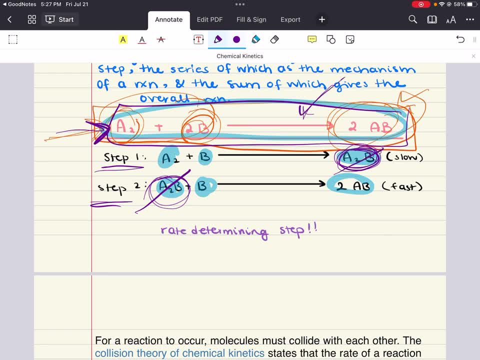 cancels out for the net overall reaction. all right, This is the net overall reaction, which is why we don't see that intermediate in the full net reaction. So let's look at step four. So this is the net overall reaction that we see. all right Now, out of these two steps, one of them is: 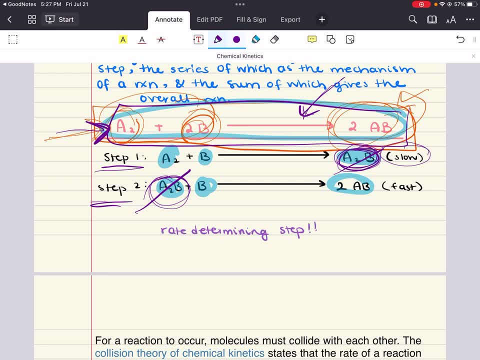 going to be slow, one is going to be fast. Your slow process or step is called your rate determining step. Your reaction can only go as fast as your rate determining step, And so this rate determining step acts like a kinetic bottleneck preventing the overall reaction. 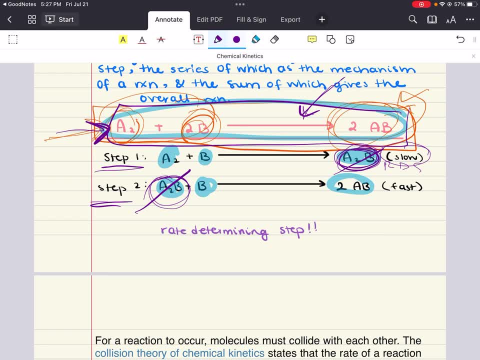 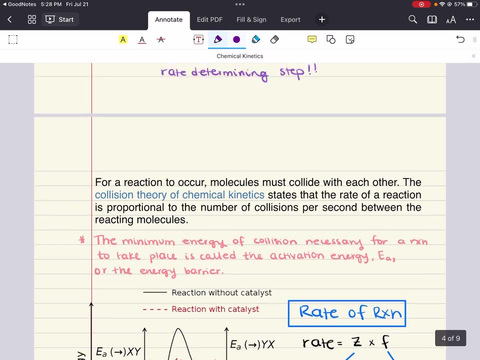 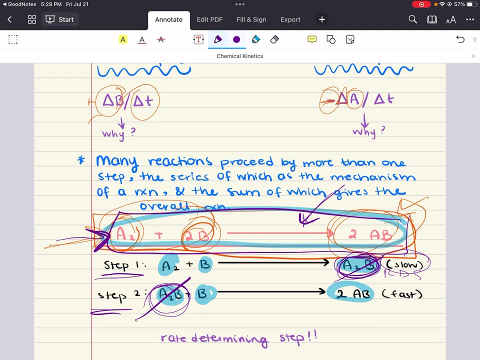 from proceeding any faster than that slowest step. all right, Fantastic. Now it's one thing to say, all right, looking back at this reaction, all right. It's one thing to say that, A2,, let me erase some of this stuff. all right, We're going to continue talking about this. 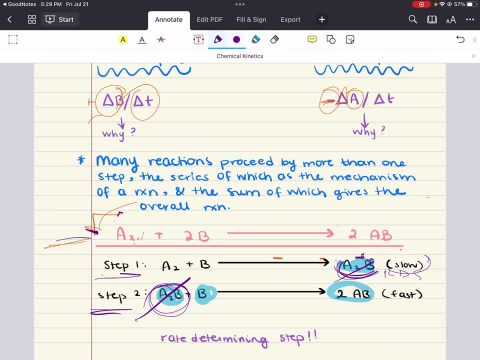 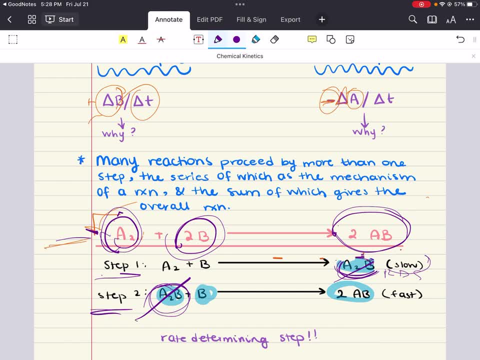 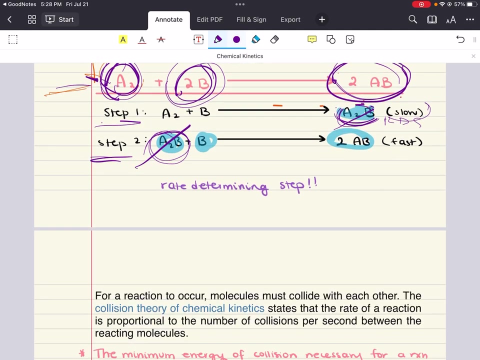 To form 2AB, And it's quite another thing to be able to describe as precisely as possible the actual interactions that are going to occur between A2 and 2B to be able to produce our AB product. all right, Various theories have been proposed to explain the events that are taking. 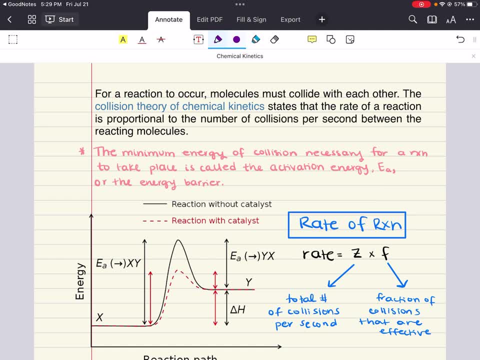 place At the atomic level through the process of a reaction. We're going to discuss, all right, the collision theory of chemical kinetics. all right, That's an important topic to be able to understand, to really fully be able to look at a reaction and understand. 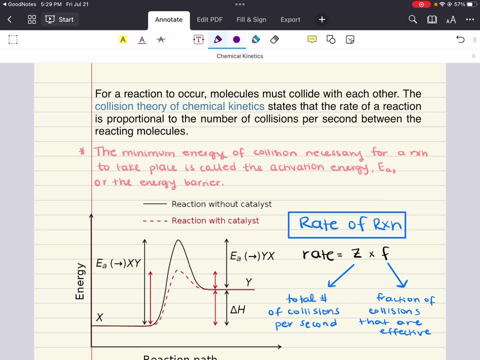 the complexities that are happening there. all right, And this is a theory that is going to be important for us to also understand for the MCAT. For a reaction to occur, molecules have to collide with each other, And the collision theory of chemical kinetics. 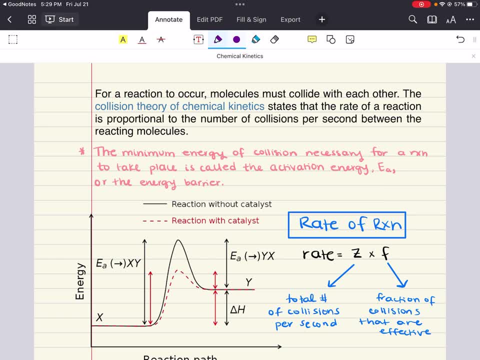 it states that the rate of a reaction is proportional to the number of collisions per second between the reacting molecules. This theory, it suggests, however, all right, that not all collisions will result in a chemical reaction. An effective collision, all right, one that leads to the formation of products occurs. 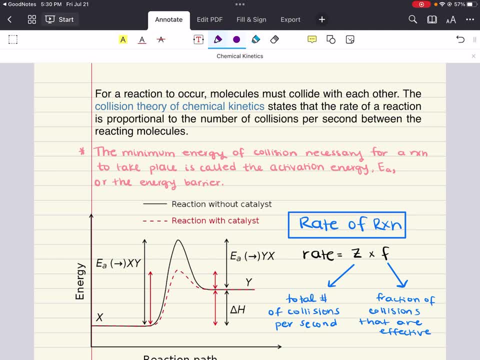 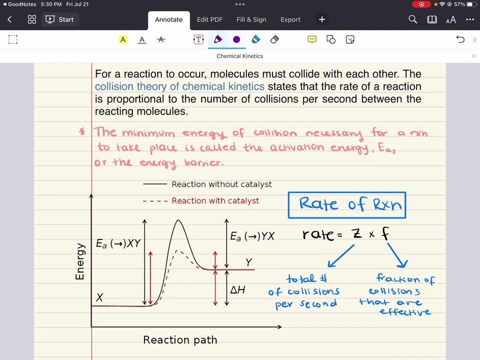 only if the molecules collide with each other in the correct orientation and with sufficient energy to break their existing bonds and form new ones. The minimum energy of a collision necessary for a reaction to take place. that is what's called activation energy. all right, or the 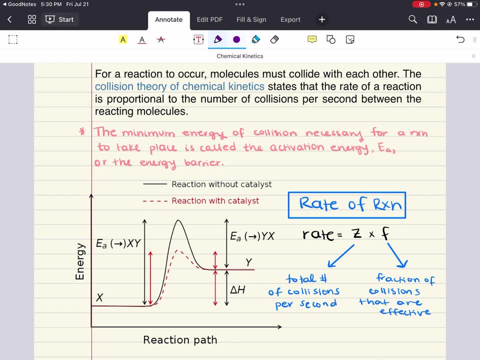 energy barrier. Only a fraction of colliding particles are going to have enough kinetic energy to exceed the number of collisions that are going to take place. So, if a collision is going to take place, only a fraction of collisions are going to have enough kinetic energy to exceed. 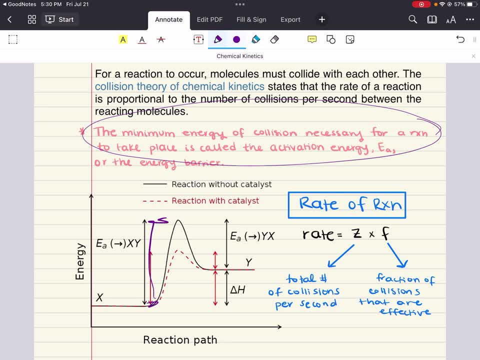 the activation energy. all right, So only a fraction of colliding particles have enough kinetic energy to proceed to exceed the activation energy, And that means only a fraction of all collisions are actually effective. right The rate of a reaction. it can therefore be: 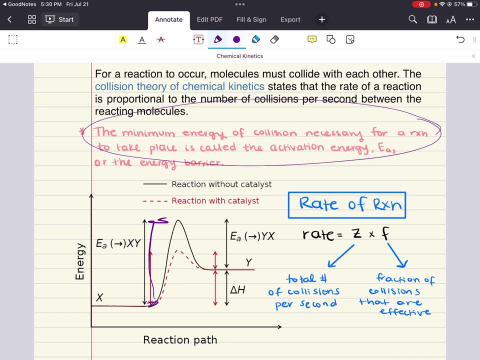 expressed the following way: all right, We can talk about rate as the total number of collisions per second multiplied by the fraction of collisions that are going to take place, So a fraction of collisions that are effective, all right, And so we see here a idea of how we can. 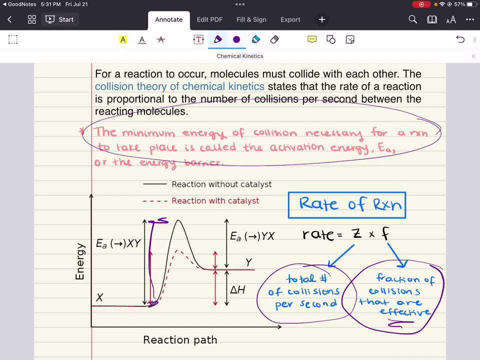 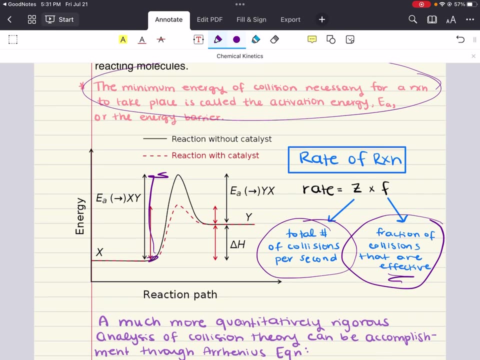 think about rate. all right, We have a way of thinking about a rate of reaction: Total number of collisions occurring per second multiplied by a fraction of collisions that are effective. give us some idea about the rate. Now a much more quantitatively rigorous analysis of this. 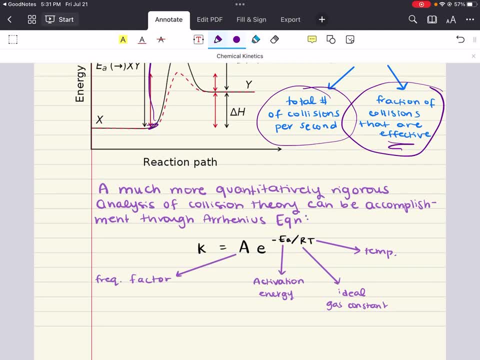 collision theory is going to give us a much more quantitatively rigorous analysis of this collision theory. It can be accomplished through something called the Arrhenius equation- all right, And it's given right here. all right. Where the rate is equal to this frequency factor, all right. 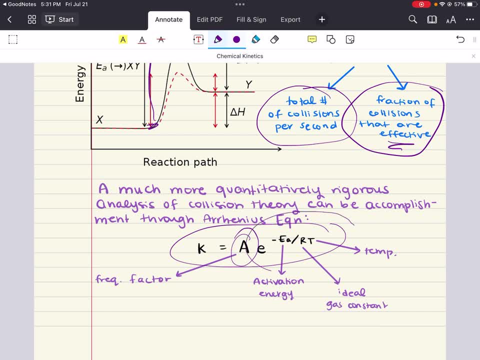 Multiplied by this exponential term, e to the power minus ea. ea is the activation energy of the reaction divided by r, which is your ideal gas constant, and temperature. all right, T. temperature in Kelvin. Now this a, this frequency factor, is also known. 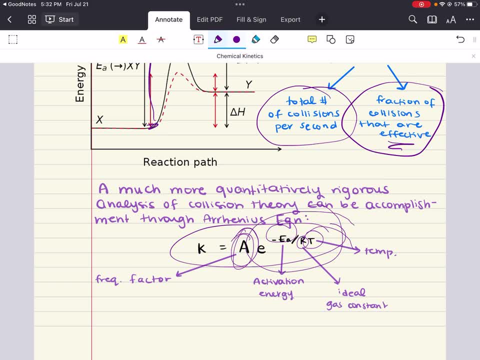 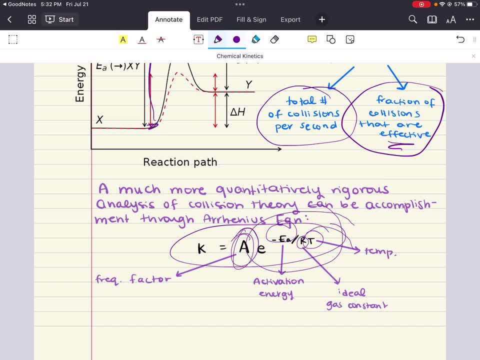 between the variables we see here and, of course, your exponent rules- because we have an exponent term here, all right- that govern this equation. they're going to be really important to understand. all right, because, while you might be tested on this equation, what's even more likely to be? 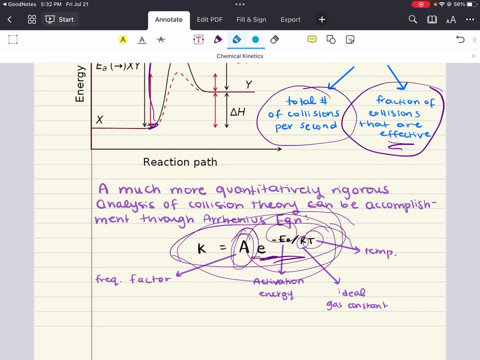 tested on is the relationship between these different variables. you see here all right, and so, for example, a simple relationship between a and k- all right- is going to be important to understand. it's kind of evident in this equation as the frequency factor all right of the reaction. 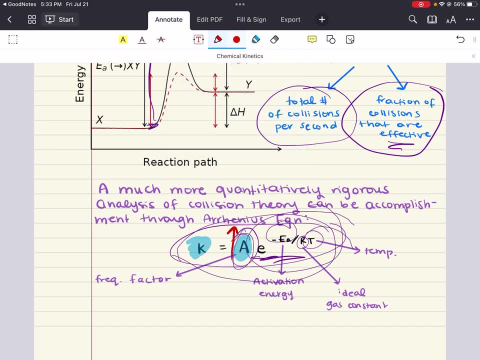 increases as a increases, what can you guess? well, you can guess that the rate of the reaction also increases in a direct relationship. all right, so they're proportional, all right. also, we can talk about temperature. if the temperature of a chemical system were to 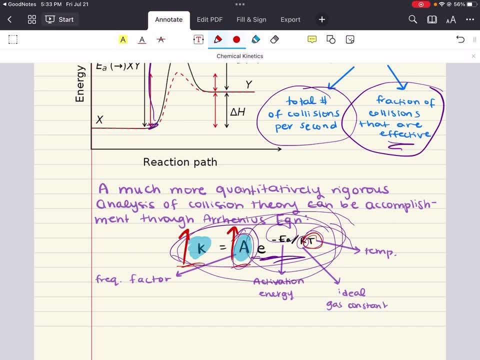 increase, all right say, to infinity. while all other variables are held constant, the value of the exponent would have a magnitude less than 1 as temperature approaches infinity. However, before assuming that the rate constant is going to decrease as a result, note: 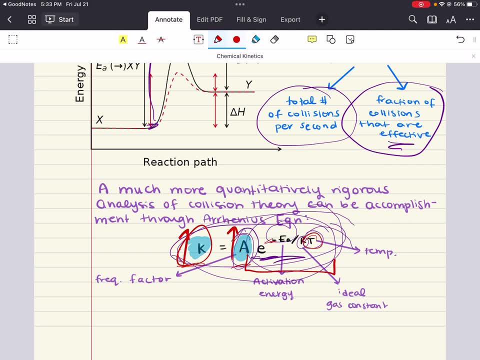 that the presence of the negative sign right here in this exponent term is important to consider. As the magnitude of the exponent becomes less negative, all right. all right, as the magnitude of the exponent gets smaller, I should say it actually moves from a more negative value towards 0.. 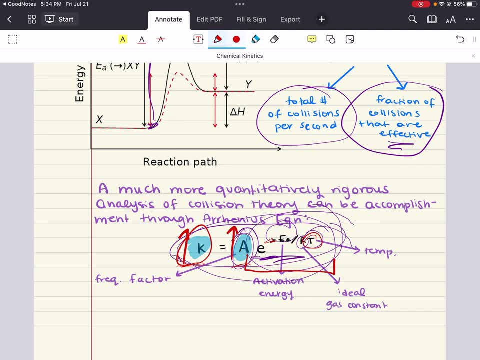 The exponent thus becomes less negative, all right, which means that the rate constant actually increases. This should make sense conceptually, because the rate of a reaction increases with temperature. all right, So here are the main points: Low activation Energy and high temperature make the negative exponent. 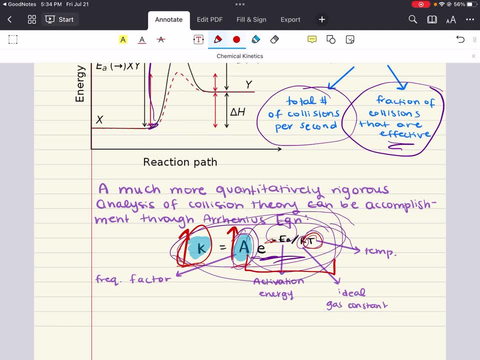 of the Arrhenius equation, smaller in magnitude, and thus increase the rate. constant k, The frequency factor, can be increased by increasing the number of molecules in a vessel, And when there are more molecules the opportunity for collision are increased. all right, Fantastic, all right. 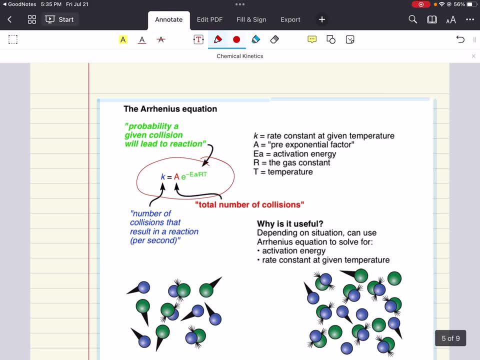 We can see that again here. all right, Here's our Arrhenius equation: K: number of collisions that result in a reaction per second. So our rate constant, k, all right, equal to a total number of collisions, our frequency factored multiplied. 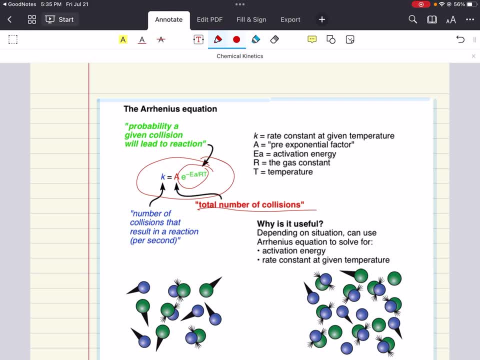 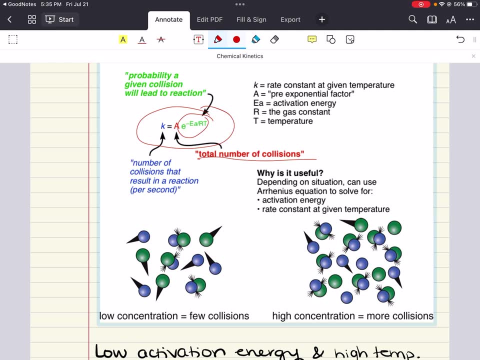 by this exponent factor which gives us the probability a given collision will lead to a reaction. okay. So why is this useful? Why is this important? the Arrhenius equation: Well, depending on the situation, we can use the Arrhenius equation. 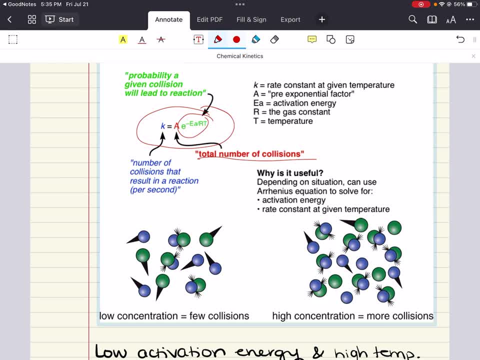 to solve for activation energy, or we can use it to solve for rate constant at given temperatures, And the way that we can think about it, especially in regards to the collision theory that we've talked about. low concentrations are gonna have fewer collisions. 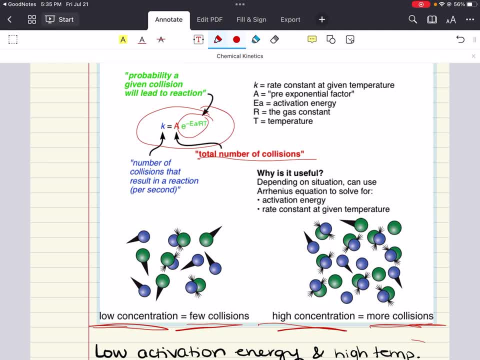 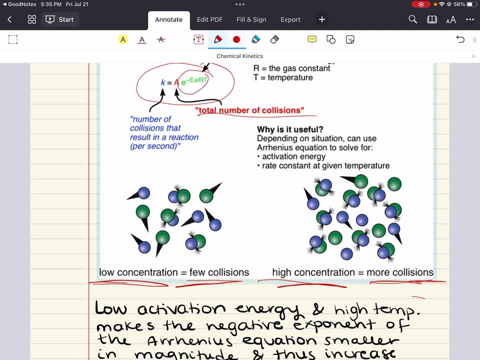 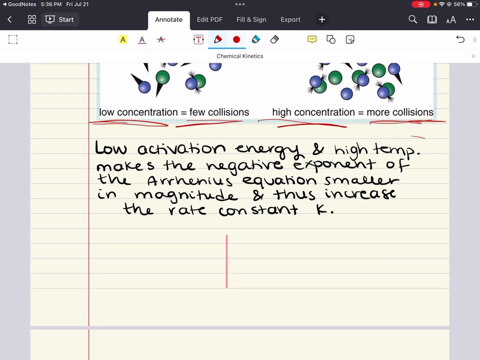 higher concentrations, more collisions, all right. And so when molecules collide with energy that is equal to or greater than the activation energy, all right. they're gonna form a transition state in which the old bonds are weakened and the new bonds begin to form. 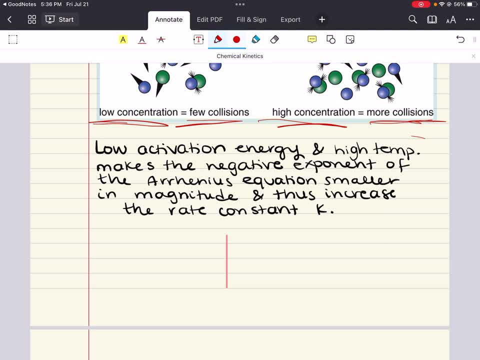 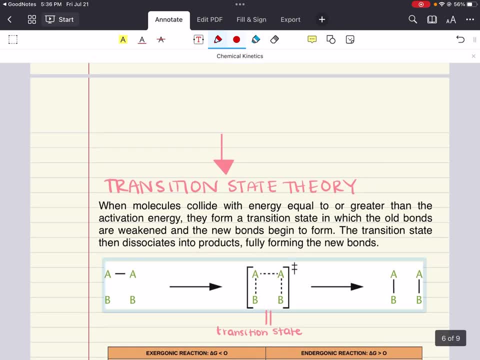 The transition state then dissociates into product, fully forming the new bonds. And so for a reaction like a2 plus 2b equals 2ab, the progress all right along the reaction coordinate which traces the reaction, which traces the reaction. 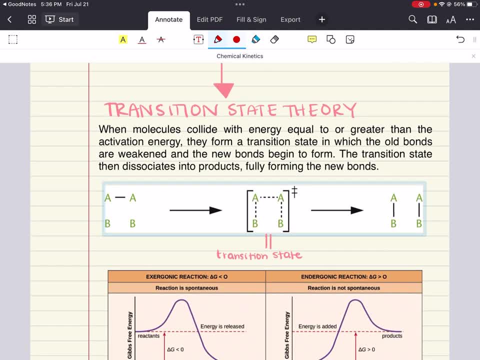 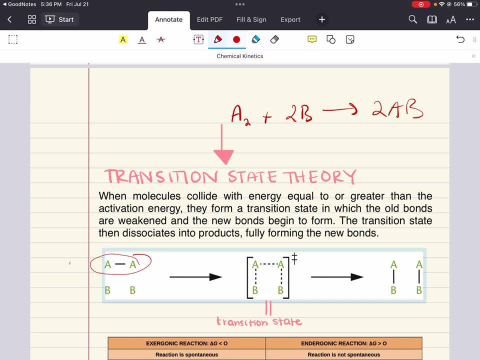 from reactants to products can be expressed and can be represented here in this figure: all right, You're starting with a2, all right, and 2b's, all right. And they interact, these reactants, and they're gonna form some sort of transition state. 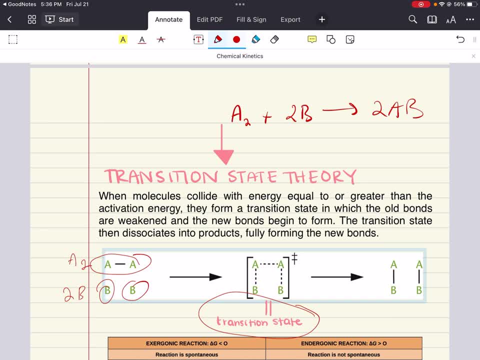 all right, they're gonna form some sort of transition state in which old bonds are weakened and new bonds begin to form, And this transition state then eventually dissociates to give us the products 2ab. all right, Let's talk about this though, all right. 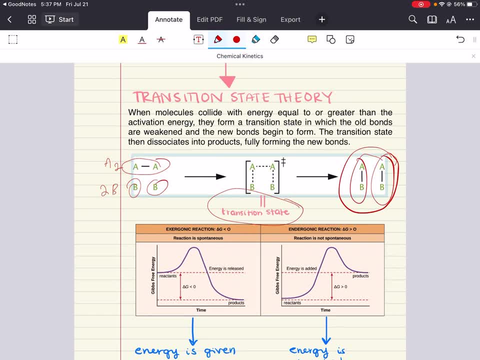 because this is really important. In the simplest sense, a chemical reaction involves the breaking of bonds in the reactants and the formation of new bonds to create the products. But this process, it doesn't just happen instantaneously. Instead, there's a certain amount of energy. 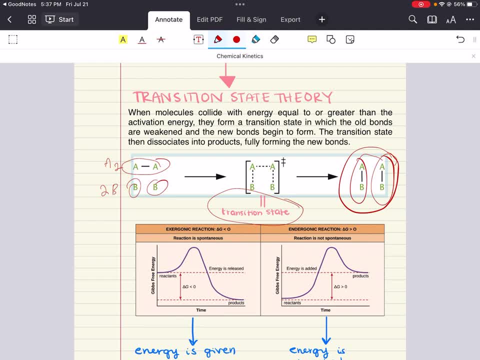 that needs to be overcome for the reaction to proceed right. that's what we call activation energy. we've seen that During a reaction when molecules collide with energy equal to or greater than the activation energy, they form a temporary configuration called the transition state or activated complex. 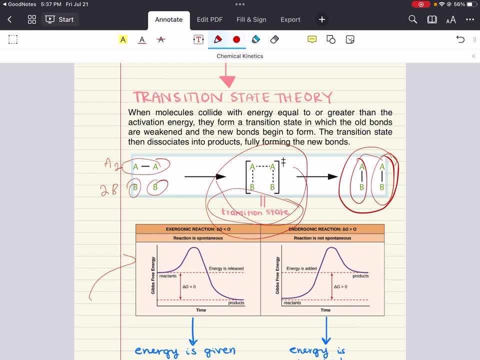 That's what we kind of saw here for our reaction, a2 plus 2b equals 2ab. all right, This state represents a particular stage in the reaction where the original bonds in the reactants have partial broken bonds. all right. 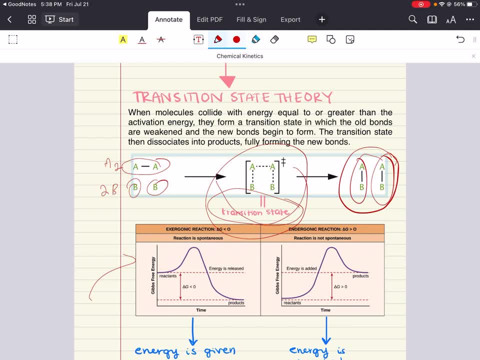 And the new bonds of the products are starting to form, all right. it is a high energy state that is unstable and it cannot be isolated or directly observed due to its fleeting existence. but it happens all right, And the transition state sits at the top of the energy barrier. 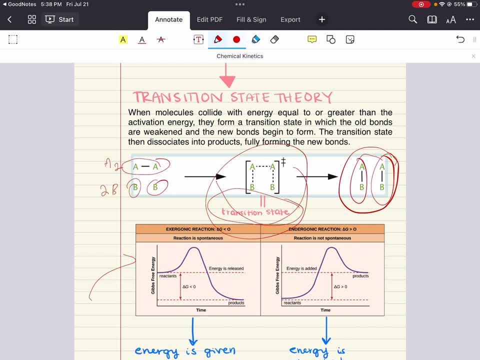 between reactants and products. The energy required to form the transition state from the reactants is the activation energy. Once the transition state has formed, it can either move forward to form products or it can revert back to reactants. all right, And so that's kind of how we want to think about it. 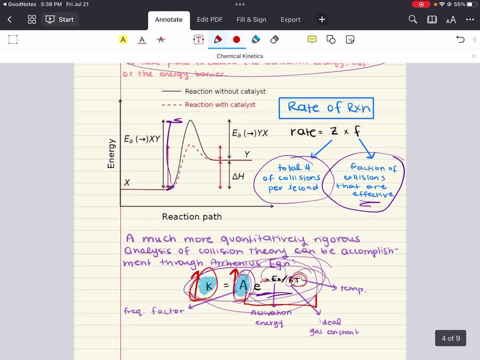 all right, We've talked about, we've talked about quite a few things. now I want to repeat so that we can make sense of this up to this point. all right, So we can make sense of it up to this point. One quick thing, though, before we summarize, right? 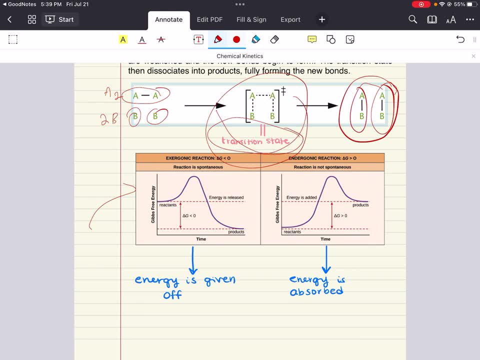 because to better visualize these concepts, right, these concepts that we just talked about, right, Chemists use this free energy diagram. We saw it previously. we're gonna look at it again really quickly. all right To graph plots. all right to graph a plot. 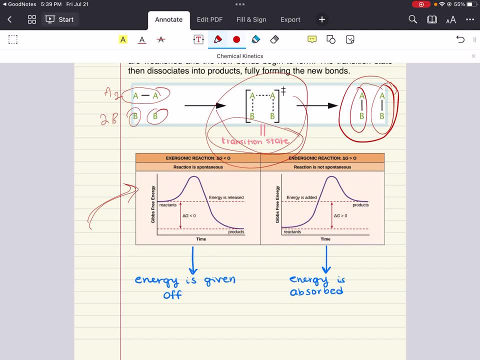 that demonstrates the change in Gibbs free energy. all right, we can plot it all right. Gibbs free energy versus time- all right, On this diagram, the y-axis represents the free energy. reactants and products are typically at different, normal, different energy levels. all right, Lower energy levels, while the transition state is going to be. 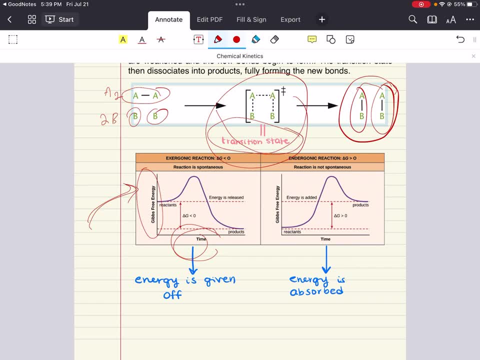 at a peak representing the highest energy level. You have your x-axis here. shows the progression of the reaction from reactants to products all right via time, And then the difference in energy between the reactants and products. that's called the free energy change of the reaction. 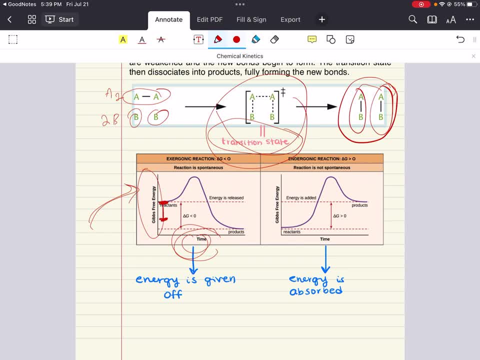 So between your reactants and products that change in energy, that's called the free energy change of the reaction. If this is negative, the reaction is exergonic and it releases energy, making it spontaneous under constant pressure and temperature. But if it's positive, then the 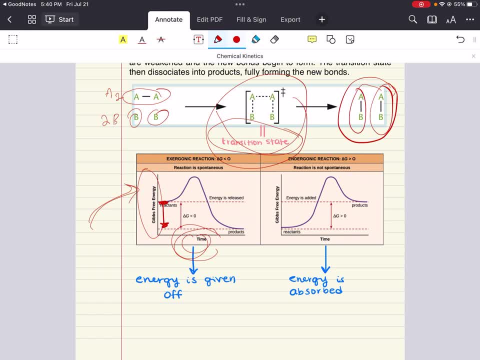 reaction is endergonic, It absorbs energy and it's not spontaneous. The difference in energy between the reactant and the transition state is called the free energy change of the reaction. So between state, that's what's known as your activation energy. all right, This is the energy barrier. 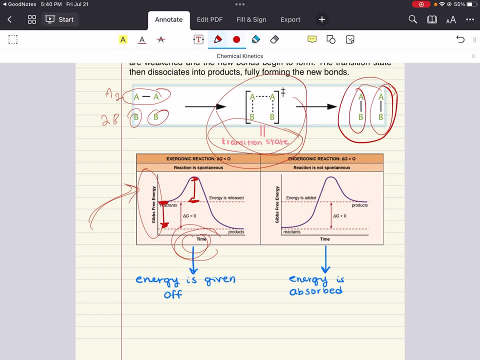 that needs to be overcome for the reaction to proceed from reactants to products. all right, And it's very important, all right. Now, all right, if your products are lower in energy than your reactants, then we're talking about an exergonic reaction. This is spontaneous. But if 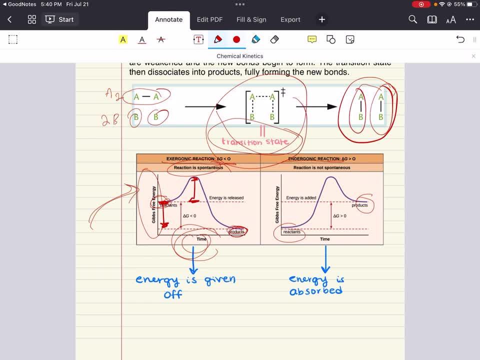 your products are higher in energy than your reactants, then we're talking endergonic and your reaction is not spontaneous. all right, So again, we covered a lot. Let's summarize this first half of the chapter. all right, Change in. 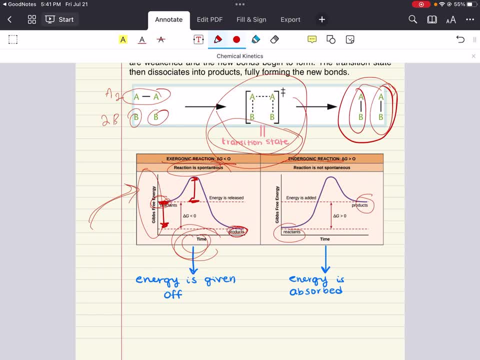 Gibbs. free energy determines whether or not a reaction is spontaneous. all right Chemical mechanisms. they propose a series of steps that make up the overall reaction. So intermediates are molecules that can exist within the course of reaction, but they're neither reactants nor 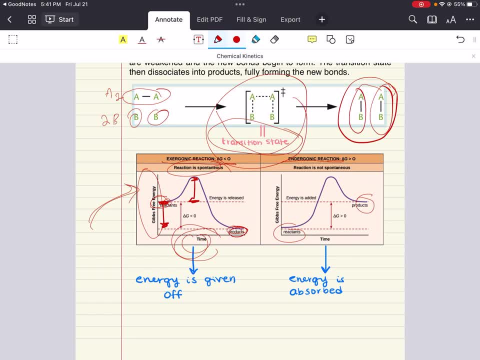 products overall. So you might not see it in your reaction. So you might not see it in your reaction, You might not see it in your net overall reaction. right, Like we saw our reaction, we saw how it can happen in step one and step two, but there was an intermediate that didn't show up in the net. 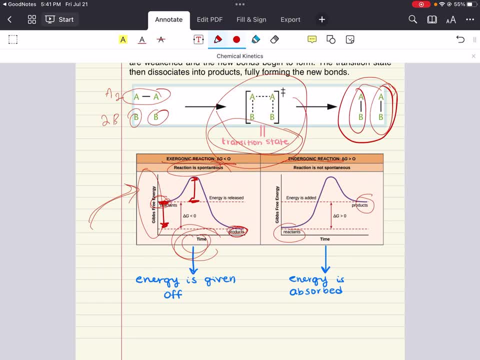 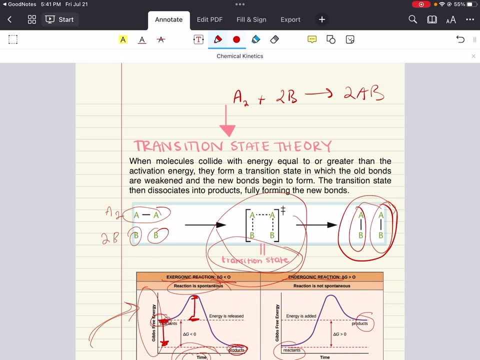 overall reaction, The slowest step, also known as the rate determining step. it limits the maximum rate at which a reaction can proceed. Then we talked about collisions theory. all right, It states that a reaction rate is proportional to the number of effective collisions between the 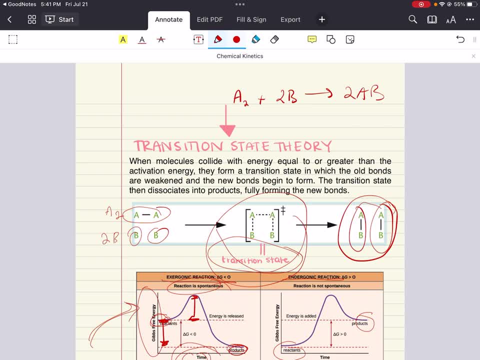 reacting molecules for a collision to be successful. So if you have a reaction rate of B, effective molecules must be in the proper orientation and have sufficient kinetic energy to exceed the activation energy. Then we also talked about the Arrhenius equation, how it is a 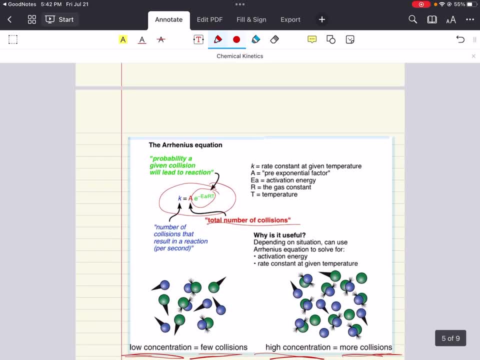 mathematical way of representing collision theory, where K, your rate constant, is equal to A, your frequency factor, multiplied by this exponent term that has activation, energy, ideal gas constant and a rate constant. So if you have a rate constant, you have a rate constant and a rate. 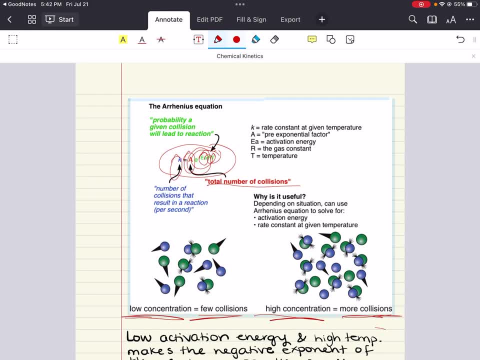 constant and temperature all right. And essentially, this Arrhenius equation can tell you the number of collisions that result in a reaction, that being equal to the total number of collisions multiplied by the probability of a given collision that will lead to a reaction. 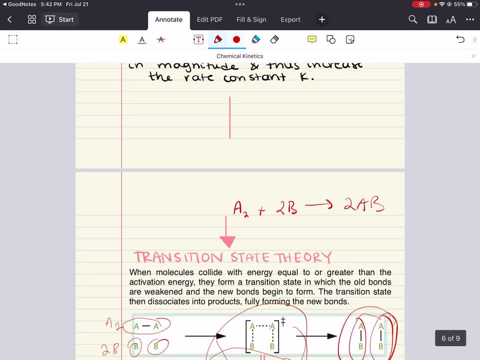 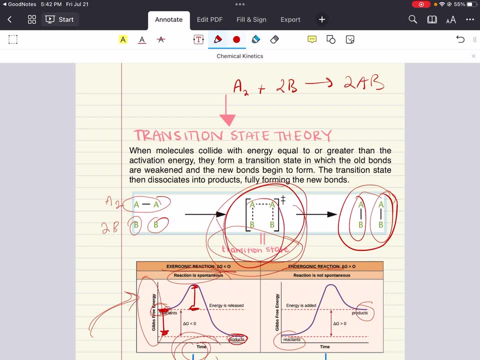 all right. We also talked about transition state theory and how it states that molecules form a transition state or activated complex during a given reaction, in which the reaction rate is partially dissociated and the new bonds are partially formed From the transition state. the reaction can proceed towards products or even revert back to reactants. The transition state is 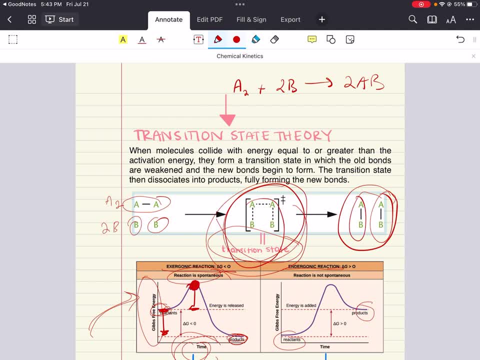 going to be the highest point. all right on a free energy reaction diagram. And lastly, we also talked about things that affect your reaction rate. Reaction rates can be affected by a number of factors. Increasing the concentration of reactants will increase the concentration of reactants. 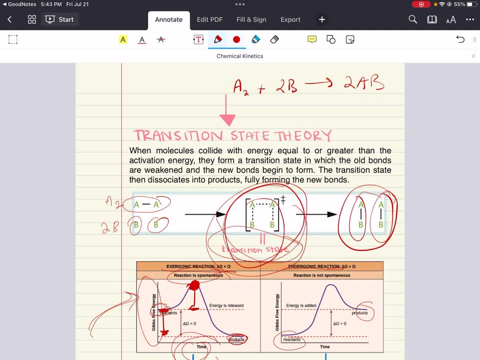 Increase your reaction rate because there are more effective collisions per time. The only exception here is a zero-order reaction, which we'll talk about later. all right, Remember, temperature also affects it. Increasing the temperature will increase reaction rate because the particle's kinetic energy is increased. Another thing is trying to change your activation. 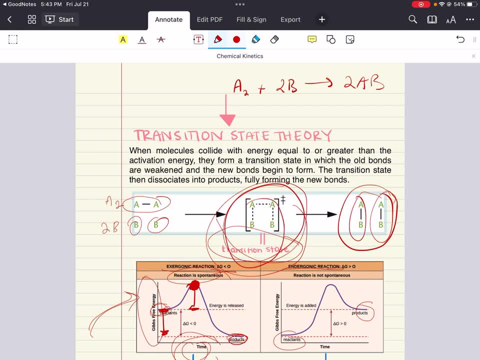 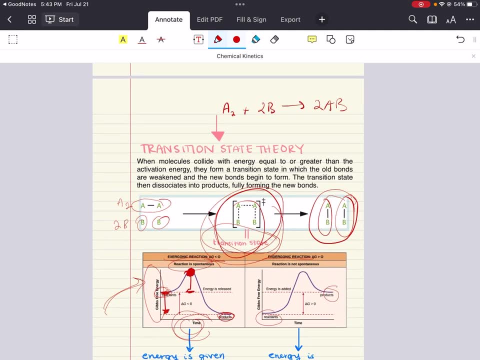 energy, and one way you can do that is through catalysts. Adding a catalyst can increase the reaction rate because it could lower your activation energy. all right, So that's a lot of information. That's the first half of this chapter. We're going to stop here. 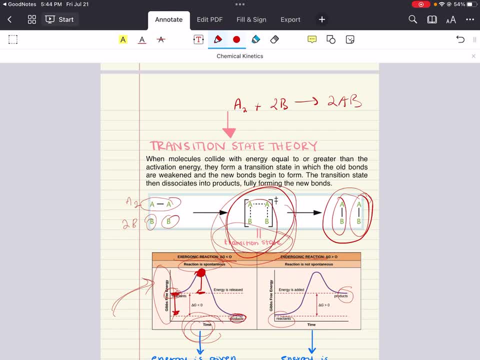 In the next video we're going to continue this chapter and talk about further rates and rate orders and the difference between a rate expression and a rate law, and then we're going to also classify chemical reactions as zero-order, first-order, second-order. 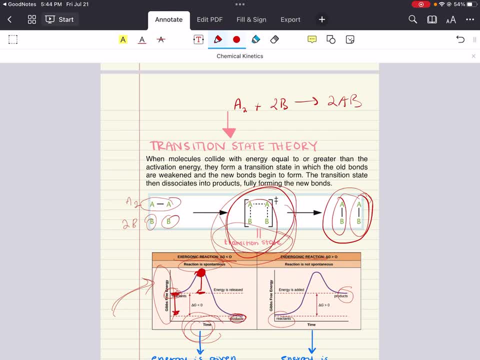 and higher-order. all right, Let me know if you have any questions. comments concerns down below. Other than that, good luck, Happy studying And have a beautiful, beautiful day. future doctors.